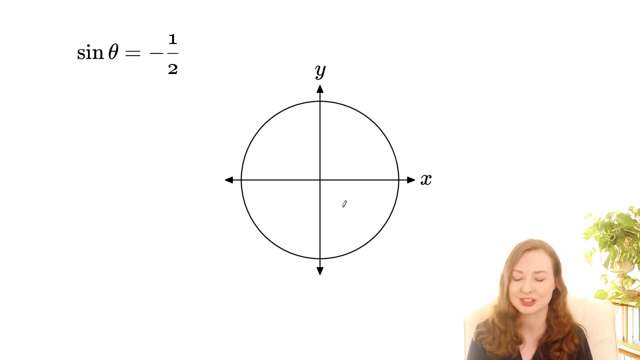 a half. So there's a really easy way to visualize this: We just go down to y equals negative a half and draw a line across there, So that represents y equals negative a half, and then the points where that intersects the unit circle. those are the angles that we're going to draw. 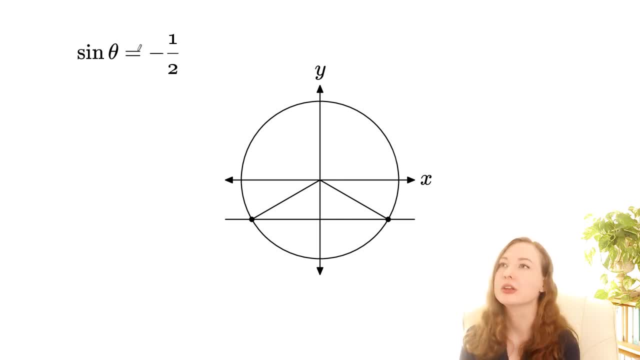 Now, because we know that this is one of the the special angles, one of the special values that I talked about in my last video. we know that this is going to be either 30, 45 or 60 degrees, So you can kind of just eyeball this. I mean that looks like 30. It's quite small, So you can see. 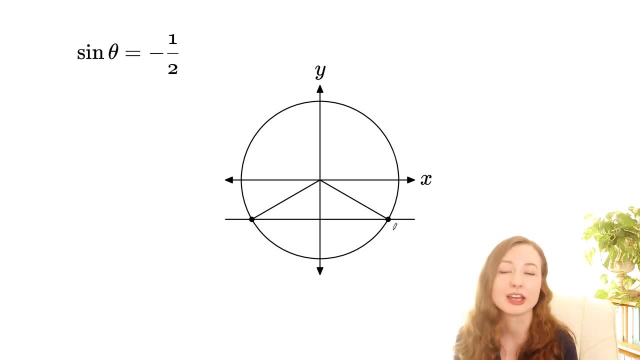 that this angle is going to be like negative 30 degrees, Or if we're working in radians, it could be negative pi on six, But there's actually a lot of different ways that you could describe that angle. You could also think of it as being 360 minus 30, so that would be 330. 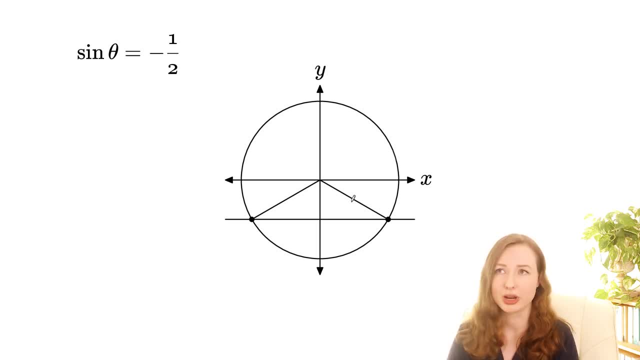 So your teacher or your test or whatever textbook is going to tell you a range of values that they want and that's going to look something like one of these four things. So if you haven't seen this kind of notation before, this just makes it more clear that we're going to want this value. 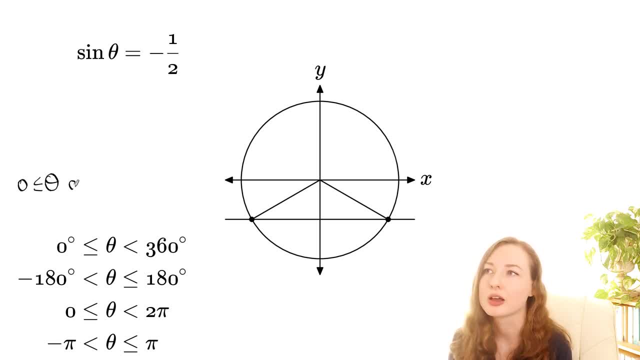 means that 0 is less than or equal to theta and theta is less than 360. So it's just sort of wrapping up those two statements into one thing, So you can think of it as just saying that theta has to be between 0 and 360.. So if they said this one one, 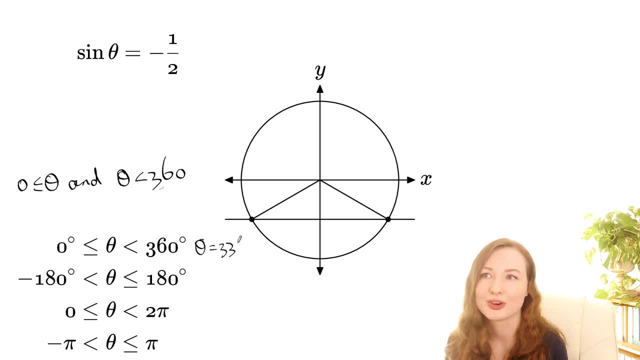 of the solutions would be: theta equals 330 degrees. for that one there, If they instead said this, then you can't say 330, because that's not within that range, because it's bigger than 180, so for that one you would have to answer theta. 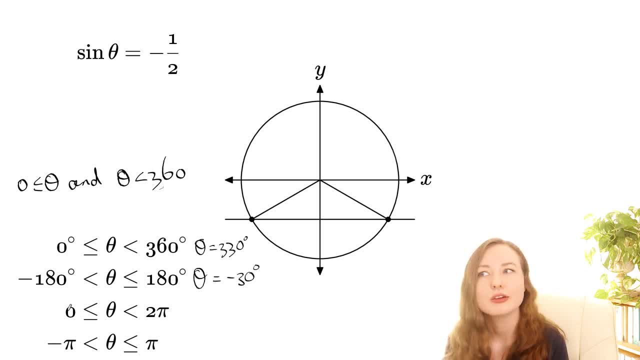 equals negative 30 degrees. If they said: let's do this one first. if they said negative pi to pi, you would say: theta equals negative pi on 6, remember that that's the same as 30 degrees. if they said 0 to 2 pi, you're. 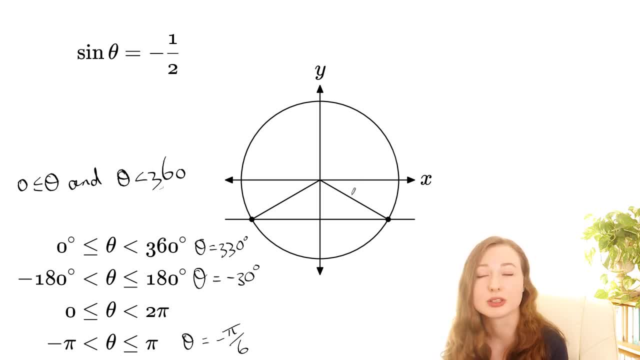 going to think that that coop will equal root within 0, because you're going to Ну будет De表 have to think of it as 2 pi minus pi on 6.. So let's work out what that makes. You can just sort of think of this as like. like, just ignore the pi's and make it 2. 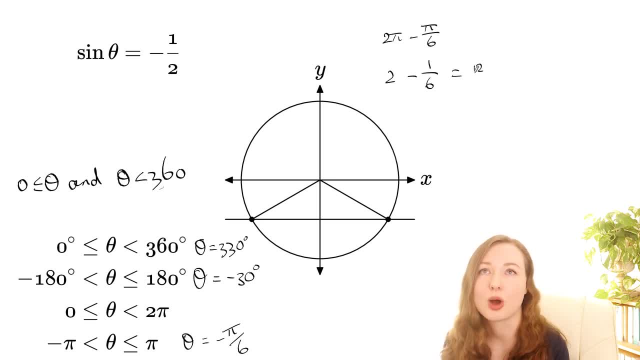 minus 1 on 6.. So think of the 2 as 12 on 6, and then that makes 11 on 6.. So you can call that 11 pi on 6.. Okay, so that's all the different ways of expressing that. 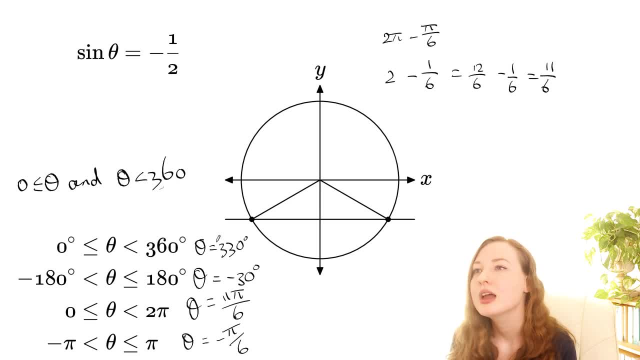 one. Now let's have a look at this one. If we're in this range, we could think of it as 180 plus 30, so that's going to be 210.. Or if we're in this range, then you would have to call that negative 150 degrees, If you find that this way is. 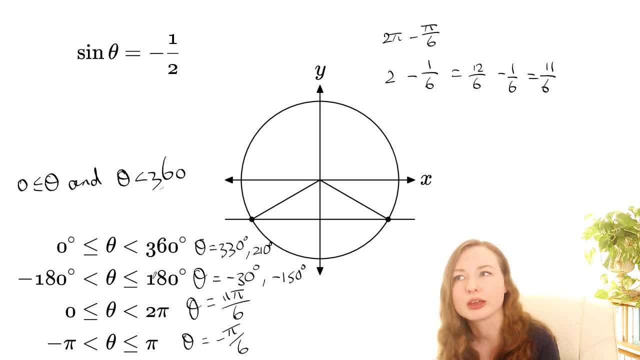 easier to think of, but they've told you this range, then what you can do is just subtract 360 from that And that will give you the negative 150. Or if you feel the other way, that it was easier to come up with negative 150, but you want to know what the answer would. 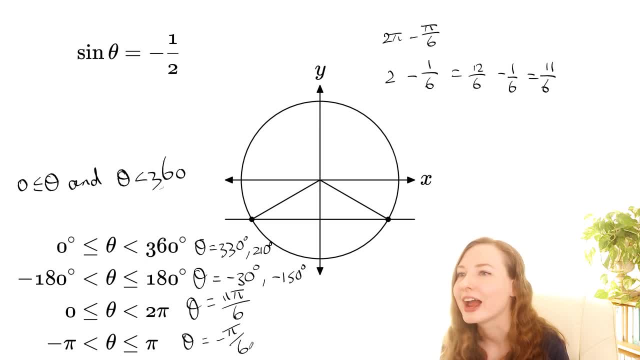 be in this range, then just add 360 to it, Okay, and then for this range it would be negative 5, pi on 6, so like negative pi, and then add pi on 6. Or if we're working in this range, you would think of it as pi plus pi on 6.. 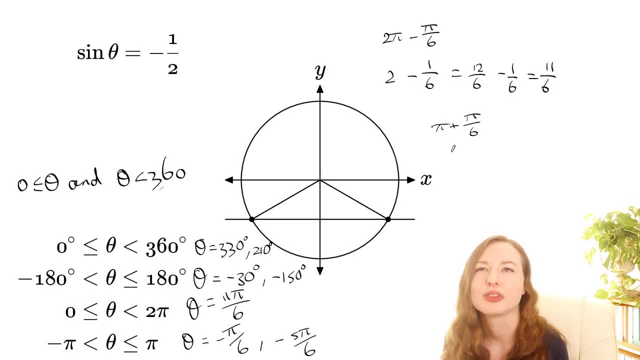 So the way to think about that is it's like 1 plus 1 on 6. And then 1 is 6 on 6. So that makes 7 on 6.. So that would be 7 pi on 6.. Okay, so that's all the ways to. 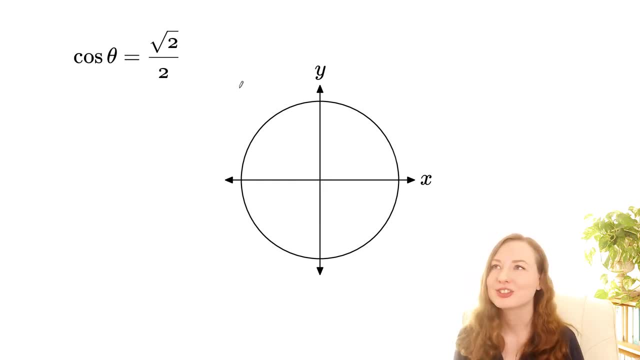 solve that equation. Let's try solving. cos theta equals root 2 on 2.. So you might remember from my last video that root 2 on 2 is approximately 0.7.. And cos theta is the x-coordinate on the unit circle. So to visualize that, let's. 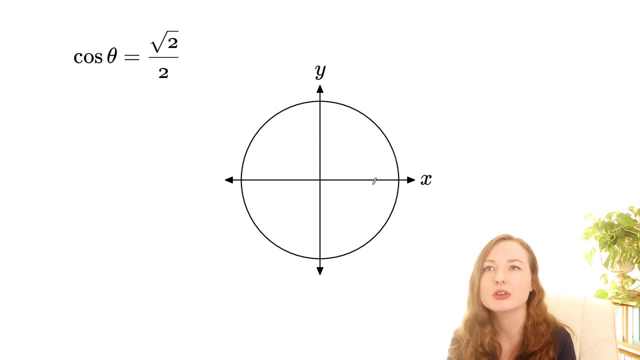 just go to x is 0.7, roughly there, and just like draw in a vertical line that represents x equals root 2 on 2.. And then the angles that we're looking for, the solutions to that equation, will be the points where that line crosses the. 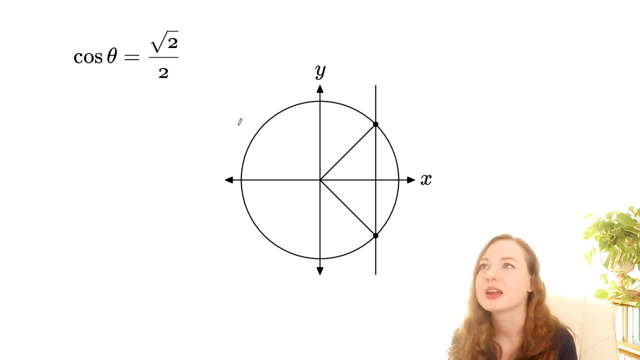 unit circle. So there and there And then again, because we know that the line crosses the unit circle. this is one of the special values that gives like 30, 45, 60 degrees. We know that this is one of those possibilities and it looks like. 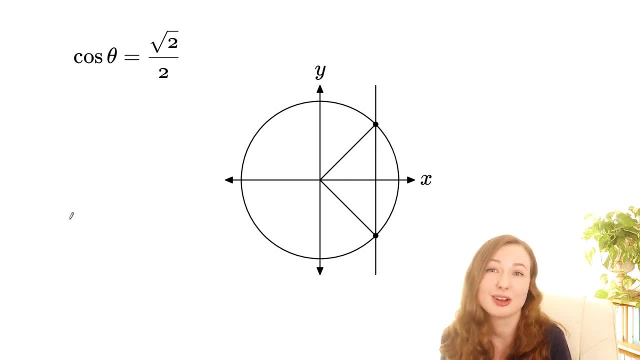 45 degrees. So you can just eyeball that and say, okay, that's, theta equals 45.. But let's have a look at the various possibilities. So for these two you can say theta equals 45 for that first one, And for these ones you can say theta equals 45.. 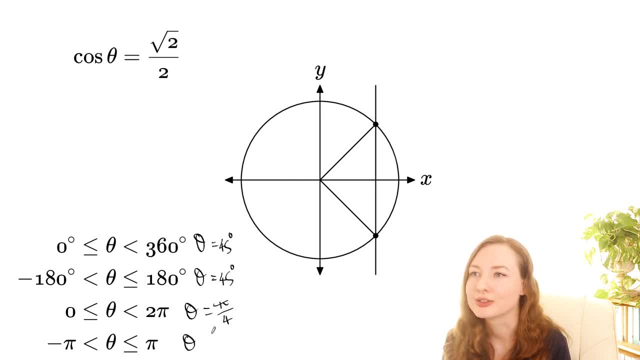 Theta equals pi over 4.. That's the radians version of 45 degrees. Now, looking at this one, you could call that negative 45, remembering that negative angles go in that direction. But if we're in this range we can't say negative 45. 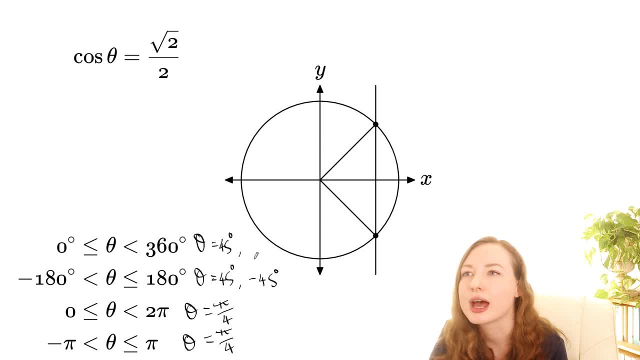 because that's less than 0. So you can add 360 to that. That gives you 315 degrees. So that's kind of like thinking of it as going around 360 and then back 45. For this range we could call that one negative pi over 4.. Or in this range: 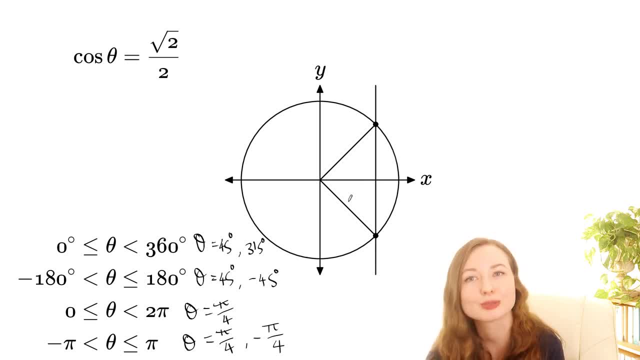 you'd have to think of it as like 2 pi minus pi over 4.. So let's work out what that would be. You can think of the 2 as being 8 over 4.. So it's like 8 over 4. 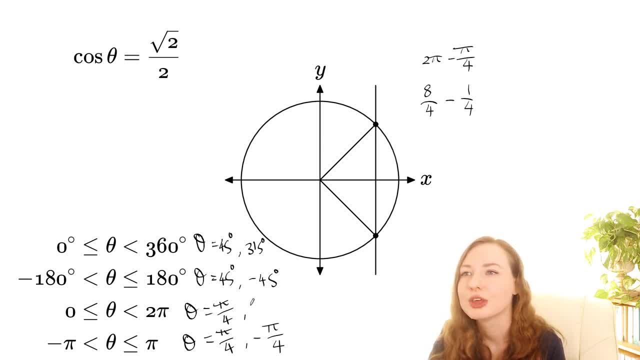 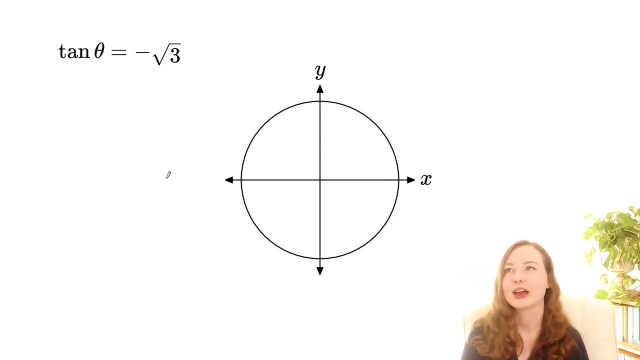 minus 1 over 4.. So that makes 7 on 4.. So this would be 7 pi over 4.. So no matter which, which range they give you, there's going to be two solutions for this equation. Let's do one with tan. So for tan theta equals negative root 3, you. 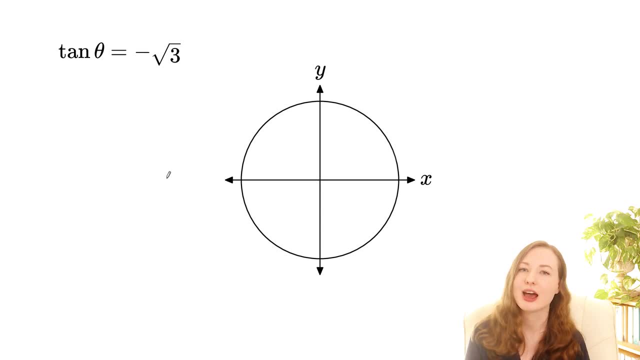 might remember from my first video that to visualize the tan what you can do is extend the line of whatever angle you have until it hits the line x, to the angle that's equal to 1.. And then the y coordinate at that intersection point gives you the tan. So what we can do to visualize that equation is draw in that. 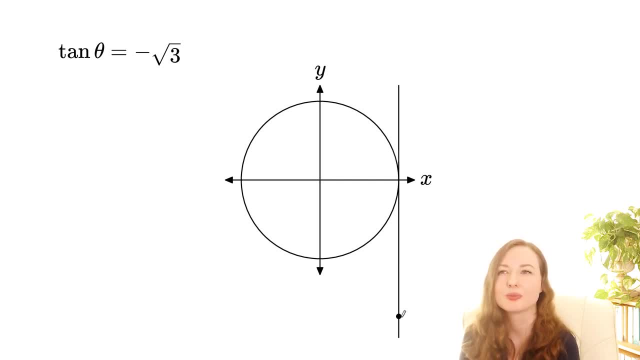 line and then negative root 3 is going to be down here. You don't really need to know exactly how big root 3 is: It's about 1 point 7.. Just know that its its magnitude is bigger than 1.. So then what we do is we draw in a line that 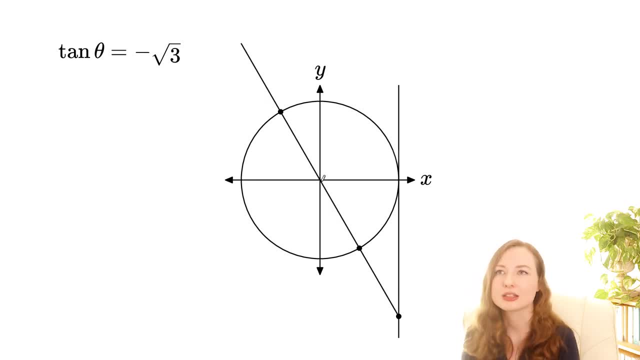 passes through this point, through the origin. So that's going to look like that. And then where that line cuts, the unit circle is the two angles that we're looking for. So, depending on what range you've been told this one again, we can just eyeball that So that 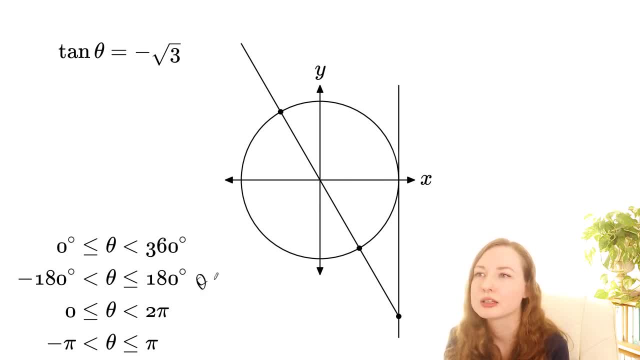 looks like 60 degrees that, so we could call that negative 60 if we're in that range. If we're in this range, then you can add 360 to that, or just like think of it as 360 minus 60, or you can even think of it as 270 plus 30 if 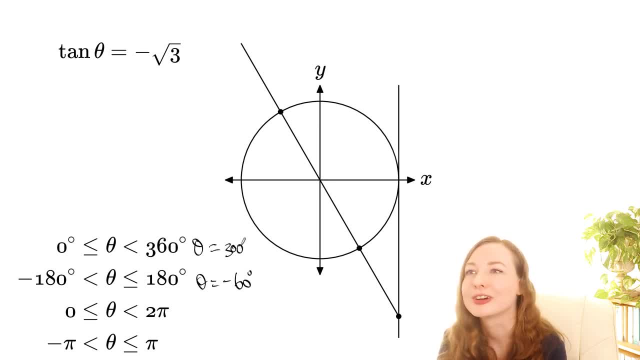 you like. So that would give you 300 degrees in any case. If we're working in radians, 60 is pi on 3, so we could say that it's negative pi on 3.. Or you could say that it's negative pi on 3.. Or if we're working in radians, 60 is pi on 3, so we could say that it's negative pi on 3.. Or 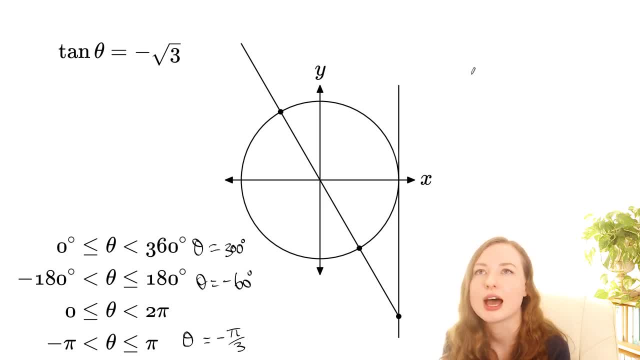 if we're in this range, then we'll have to think of it as 2 pi minus pi on 3.. So think of the 2 as 6 on 3.. 6 on 3 minus 1 on 3, that makes 5 on 3.. So that: 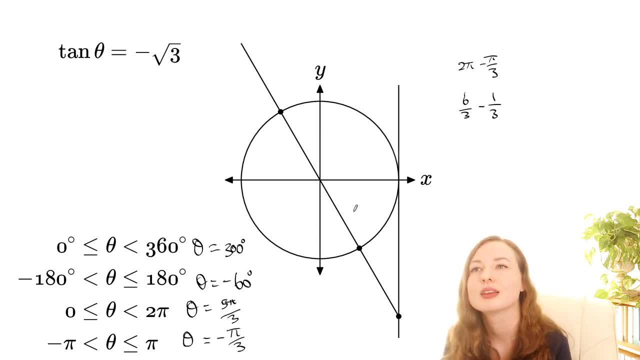 would be 5 pi on 3.. Okay, so that's that one done. Now for this angle, in either of these two cases you can just call that 120 degrees, Because they're they're in both of those ranges And for the radians we can. 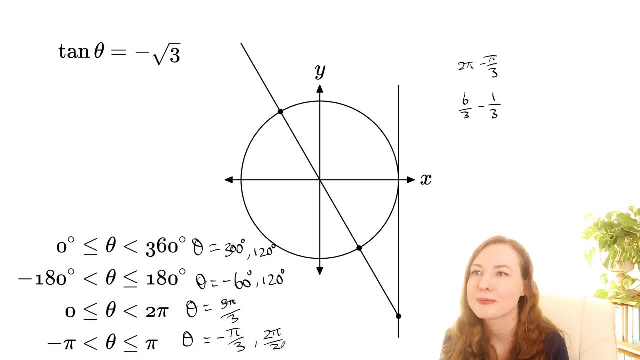 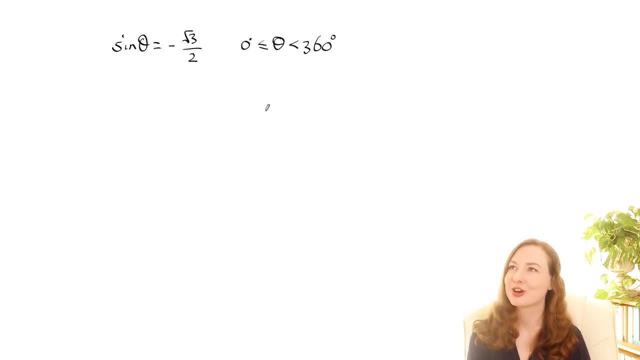 call that 2 pi on 3, or, yeah, same same for that range: 2 pi on 3 for that one as well. Okay, so that's all the solutions to that equation in those ranges. Alright, let's have a go at solving this equation. Sine theta equals negative root 3 on 2. 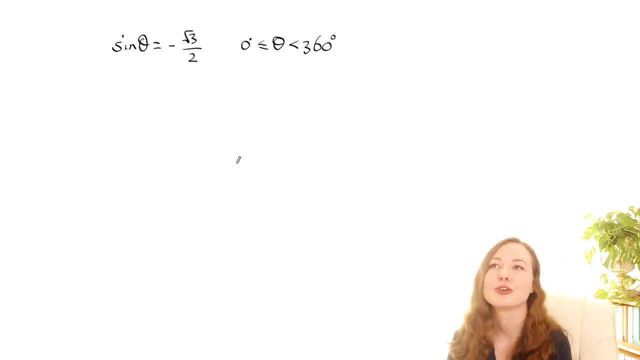 for theta between 0 and 360 degrees. So the first thing that I would do is draw the unit circle and then remember that sine is the y-coordinate. so we go down to negative root 3 on 2, which is about 0.9-ish. So down there and then we 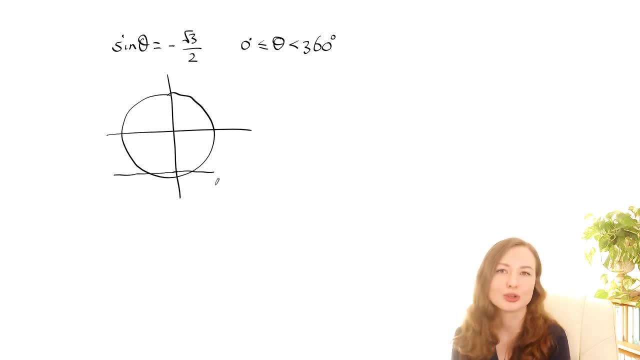 just draw in that line. y equals negative root 3 on 2, and then these two points where it cuts the unit circle. those represent the angles that we're interested in. So you can just, you can just see that that's roughly 60 degrees, Like you don't. 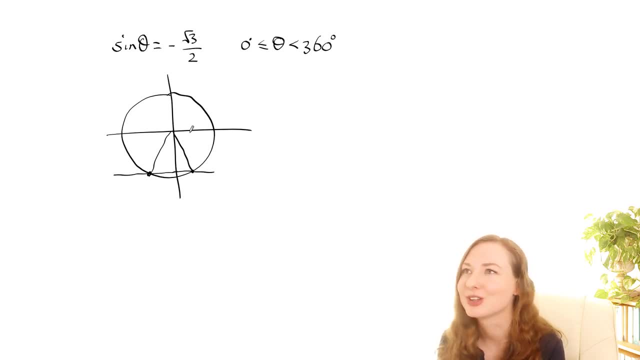 even have to put any effort into remembering special angles or anything. you can just see it on the diagram. So you can think of that as 180 plus 60, so that would be 240 degrees, And then for that one you can think of it as 270. 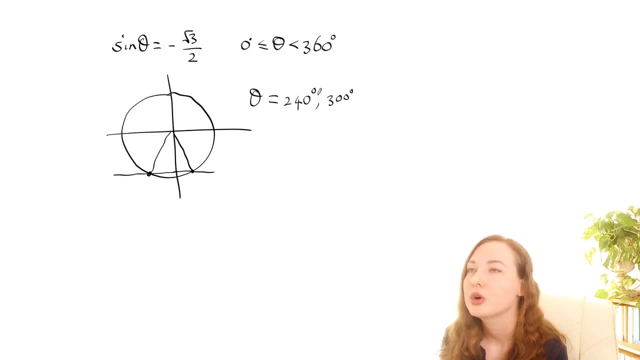 plus 30,, so that would be 300. Or you can think of it as 360 minus 60, and that also gives you 300.. So that's how you solve that one. Let's have a go at solving cos. theta equals a half for theta between negative. 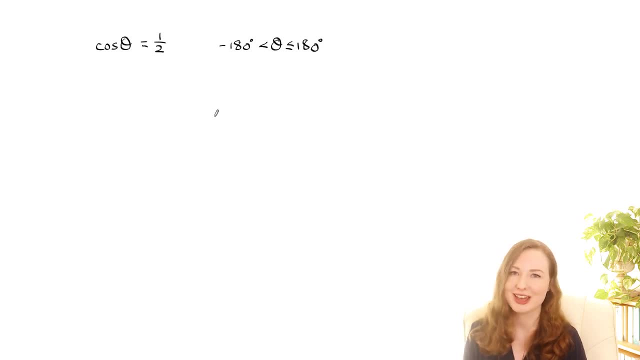 180 and 180.. So if you feel like you can figure this out, then pause the video here. Now, the first thing that I would do is draw the unit circle and then remember that cos is the x-coordinate? so we go to: x equals a half, which is around there, and 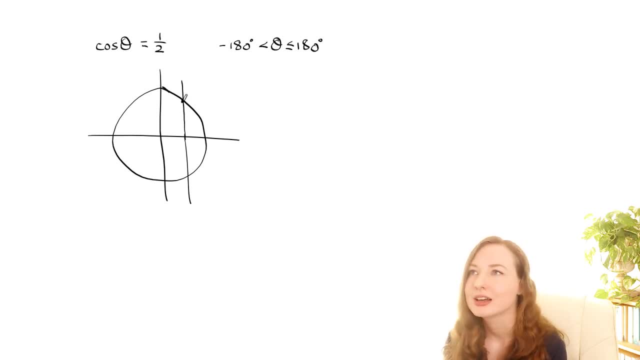 just draw in a vertical line Like that, And then these are the two angles that we're looking for, and you can just see that that looks like 60 degrees. So we're gonna get theta equals 60, and then this one you would call negative 60 degrees. We can't call it 300. 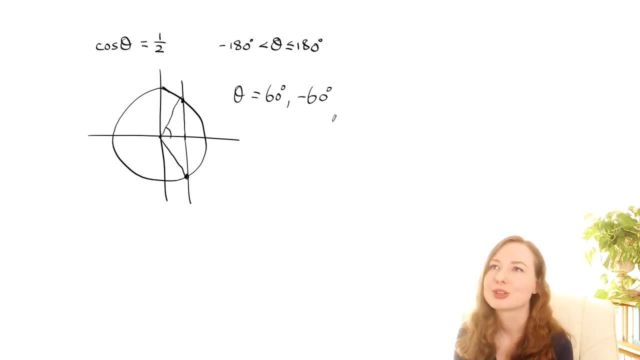 degrees, because that's not in that range. So those are the solutions to that one. Let's try tan theta equals negative 1 for theta between negative pi and pi. So pause the video here if you want to figure it out for yourself What I would. 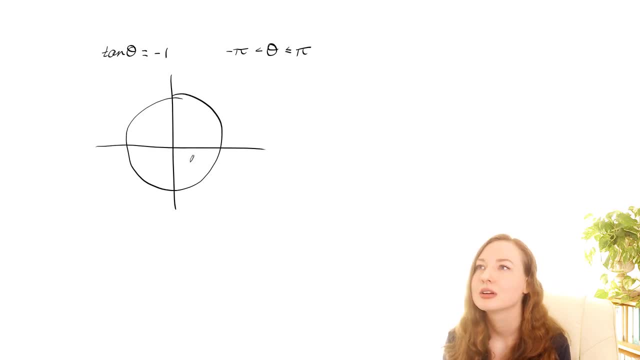 do first is draw the unit circle. It doesn't even have to be too accurate For tan. what you want to do is draw in a line x equals 1, and then go down to y equals negative 1 on that line. So just remember that, because it's the unit. 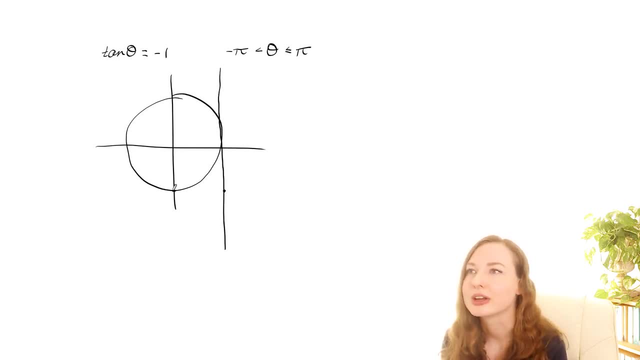 circle. that means that its radius is 1.. So this is down here at negative 1. It needs to be level with that. And then we just draw a line that goes through here and through the origin, And then you can see that that looks like 45 degrees, which is: 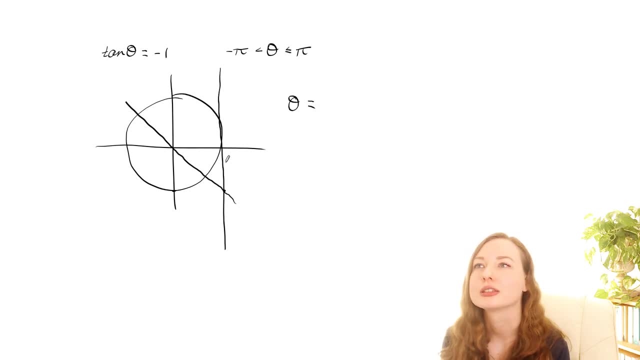 pi on 4 in radians. So you can say this one would be negative pi on 4, and then this angle would be 3 pi on 4.. So those are the solutions to that one. All right, let's have a go at sine. theta equals 0 for theta between 0 and 360.. So first thing, 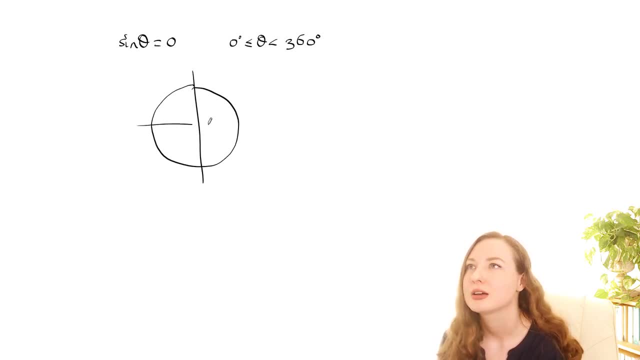 I would do is draw the unit circle. Now we want the y coordinate to be 0. So you might be a bit confused about whether this line should be vertical or horizontal. What you can do is maybe think of it as like y equals 0.0001 or something. So just go up. 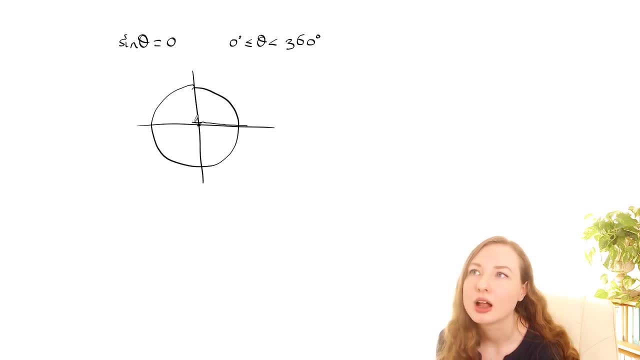 a little bit. So it's going to be going 0.0001.. So it's going to be going along like that, But you've got these two intersection points So we could say theta equals 0 degrees or 180.. Now, if they said this exactly, then 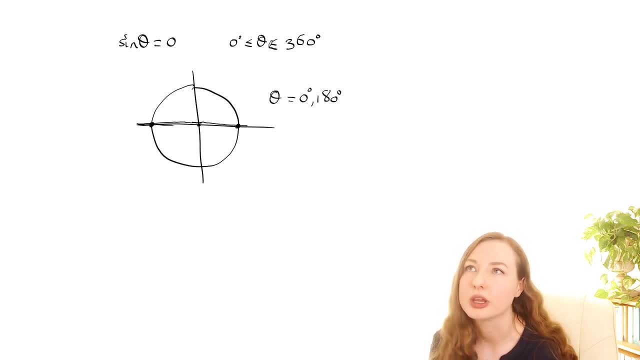 that would be it. If they said less than or equal to 360, then you would also have to include the 360 degrees, because that's there as well. So that would actually have three solutions if they said less than or equal to 360. 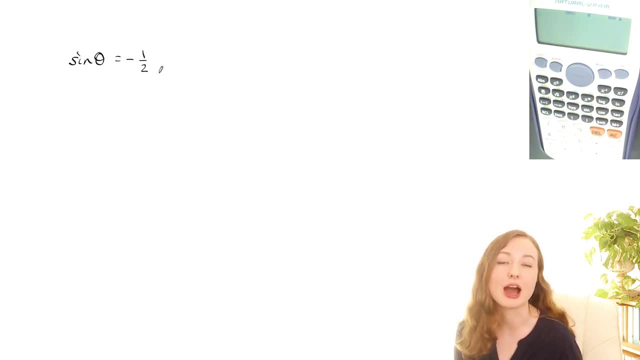 Now, if you're not confident about your answers, you can always check them on the calculator. So let's say you were solving sine theta equals negative 1 half, and you thought that maybe negative 30 degrees was the solution. You can go to your calculator. Make sure that. 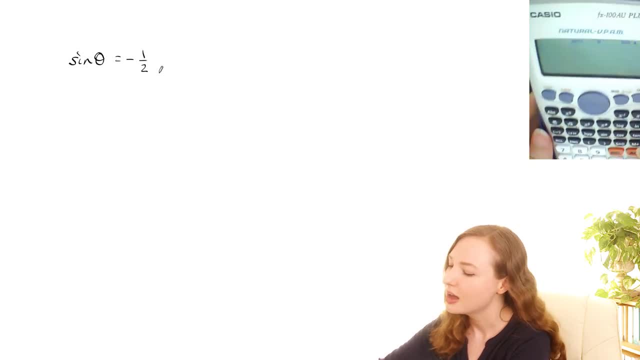 it's in degrees mode, so that's what that little d means, And you can just type in sine: negative 30,, hit equals, and it says negative 0.5. So that one's correct. If theta equals 0.5,, then that's correct.